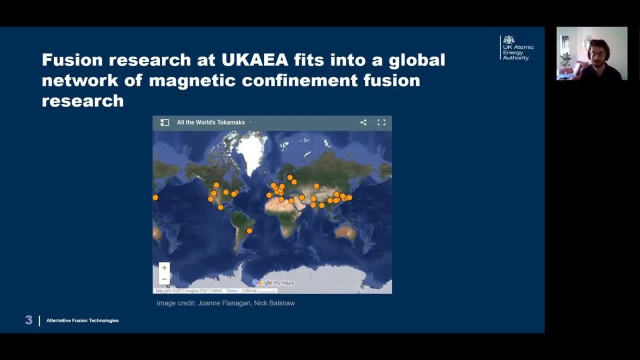 there's been 185.. So this map here shows a bunch of different operating tokamaks around the world And a lot of our research is actually done in collaboration with these labs. Many of them are government-funded labs, some of them university labs as well, And I like to say that fusion 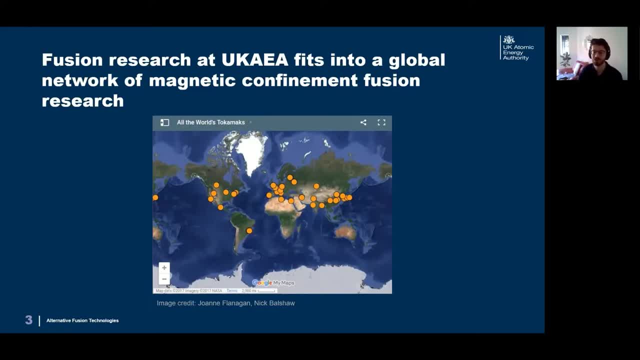 reactors are a bit like theme parks in that all of them have got something that breaks some kind of record. So JET, our largest reactor, is the largest in the world And we've got a lot of records out there that say it's the most powerful and is the most powerful, the only one that can. 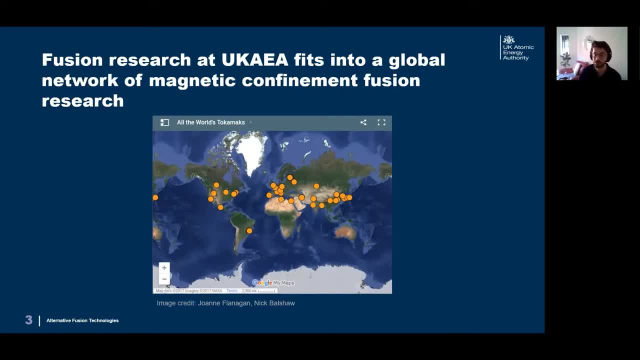 operate with tritium fuel at the moment, But there are many other records out there, So JT60 claims a lot of others, including the highest triple product, So that's the best conditions for fusion. The longest high confinement plasma has gone back and forth between KSTAR in South. 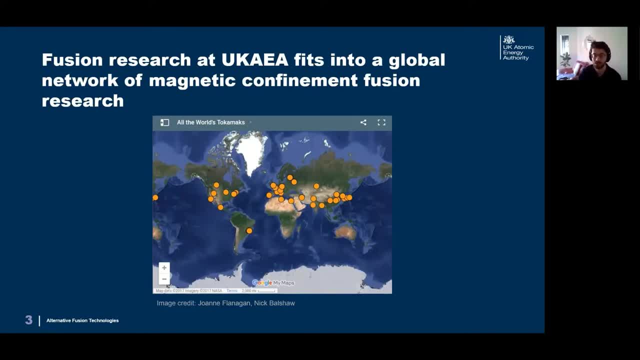 Korea and EAST in China, both of which are superconducting tokamaks as well, So that's something we just don't have. on JET, We have conventional tokamaks, So that's something we don't have. on EAST, We have conventional tokamaks, which are just a bunch of copper magnets. 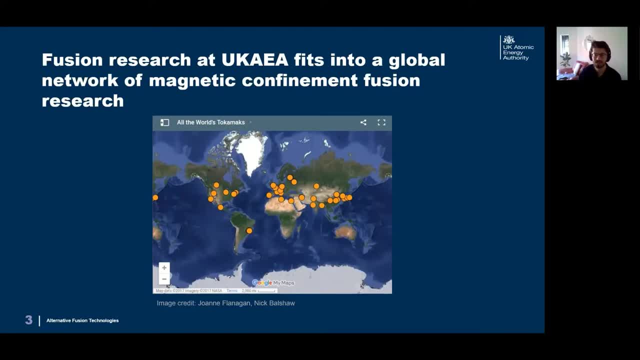 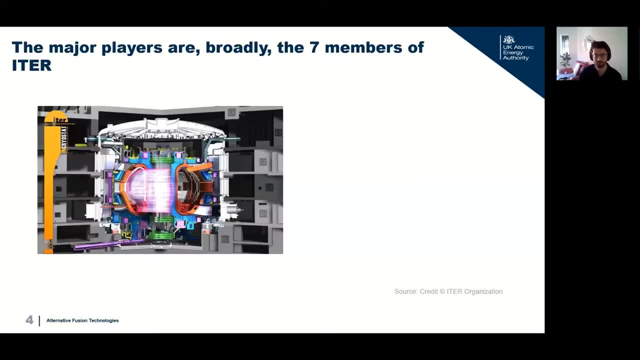 whereas these are using superconducting magnets, so could just run for much longer. Of course, on this list of 185, a lot of those are smaller ones. So who are the main players? Which are the main ones we're interested in? Broadly speaking, the major players are the seven members of ETA. 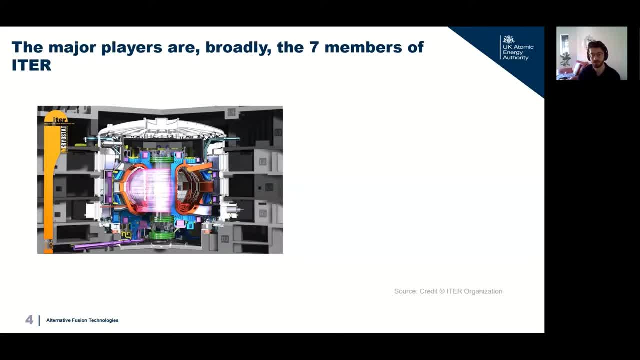 So ETA being built in the south of France at the moment will be the largest tokamak ever built, around 10 times the size of JET, And its seven members are China, the E and China, And China's main players are the EU, India, Japan, South Korea, Russia and the USA, So 35 countries total. 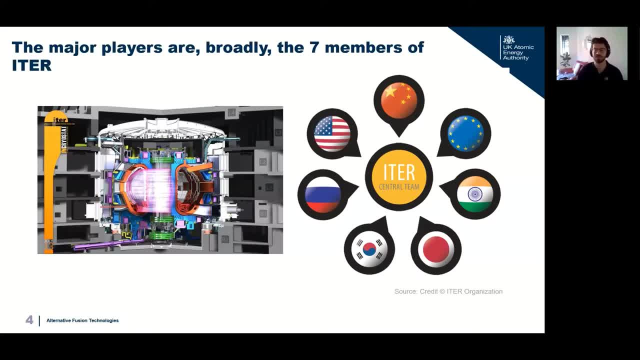 representing about half the world's population and, I think, over 80% of its GDP, And each of these countries operates their own tokamaks as well, And we need results from all of these to build together our cumulative understanding to go into ETA. We just simply can't do the full range of 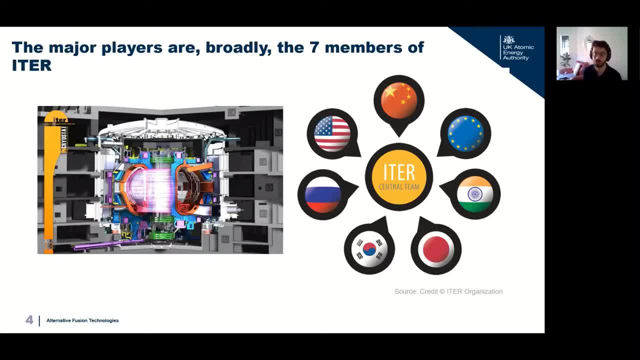 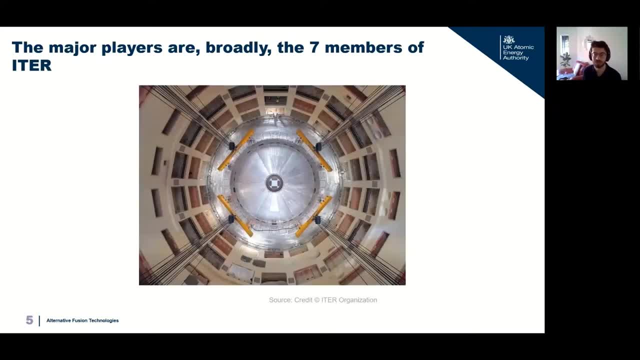 experiments required to get all the knowledge in order to run ETA just by using JET at last, Though they are a very big part of the puzzle, This is a part of ETA being installed. a few weeks ago, Remember I said how big it was. This is the cryostat base, which is the bottom of the container. 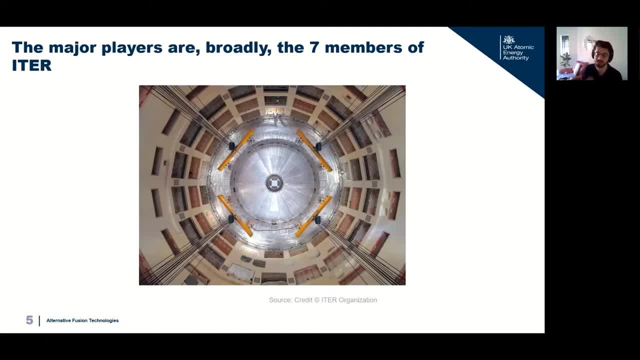 basically that all of the magnets will sit inside and the search of the vessel sits inside. That is a 1,250 tonne part being lowered in. It is absolutely huge. Here is a picture of it from underneath And these are people there to give you a sense of the scale. 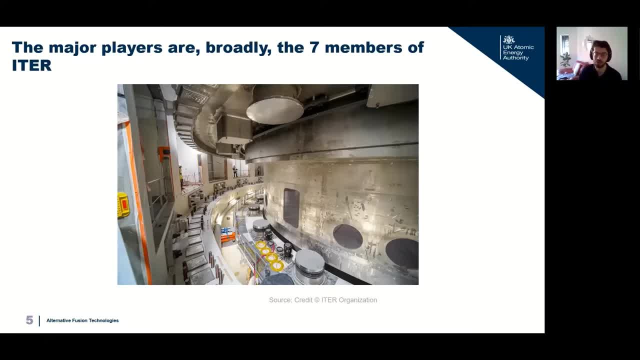 So it's absolutely important that we get things right for ETA. You can't be building something this big on a gamble, So it's absolutely essential that we have a range of different results from a range of different tokamaks around the world. But when we talk about magnetic confinement, 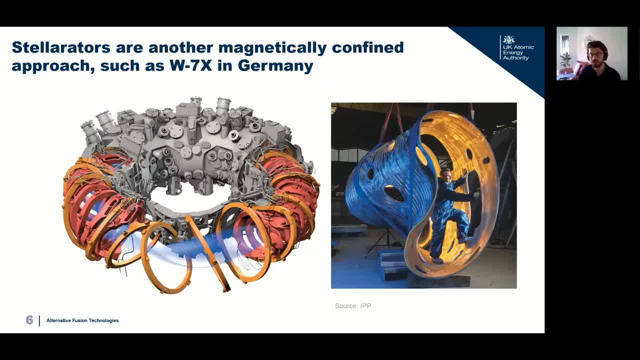 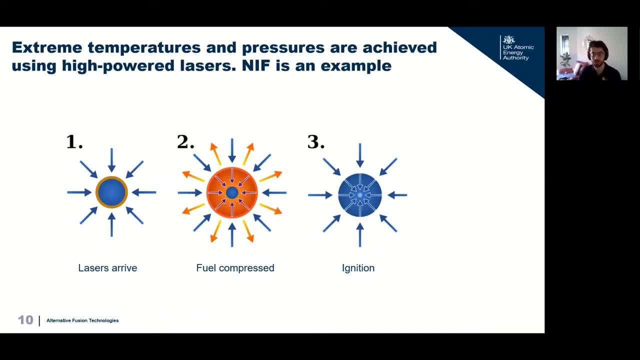 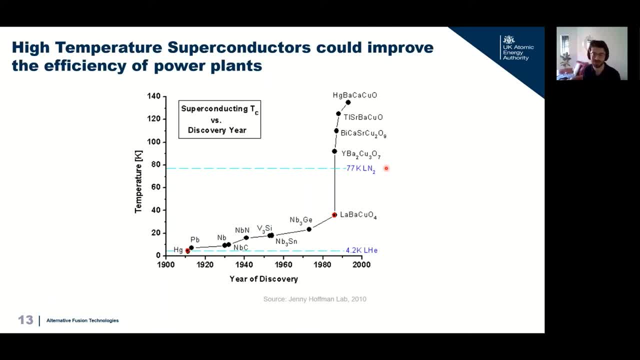 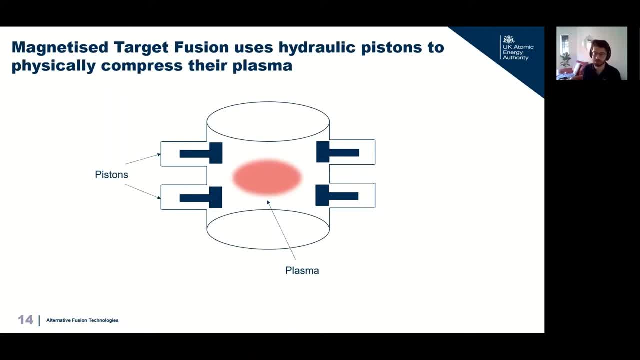 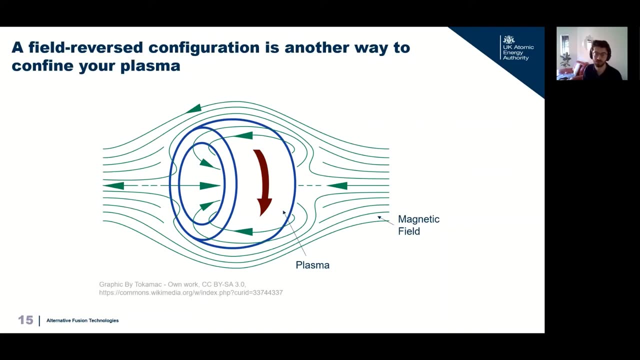 different way of doing things. Studio, Studio, that it's like basically blowing a very hot smoke ring. So this blue ring shape here is our plasma and it's blown into shape and it's sort of self-stable, rotating in position. like that The shape of the magnetic field is not worth worrying about too much, but an important 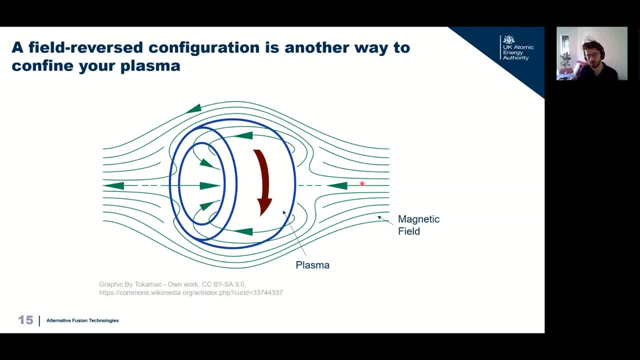 distinction is that there's no center column going through the middle here, So you don't have to have that large center column, like you do on jet, or that very small one like we do on Mars, and that can allow you to configure things differently. The benefit of a field reverse. 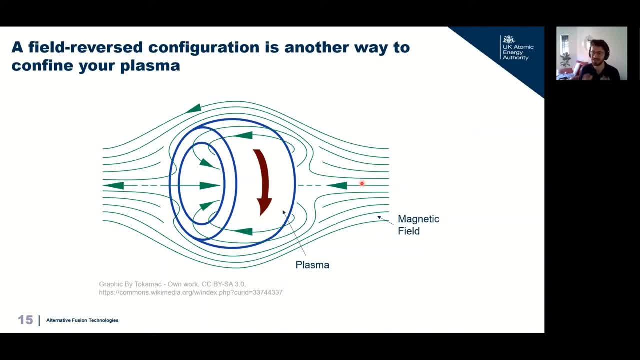 configuration from a physics perspective is you can get much higher densities in the core of the of that plasma ring- So good for the triple product, as we recall. and those higher densities could mean that it's better for harder to use fuels. So we've talked a lot about doTERRA and 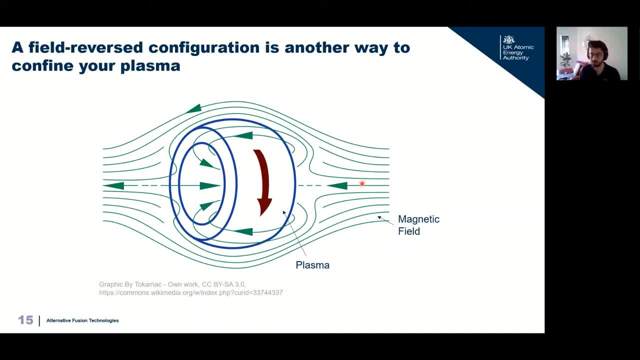 tritium and all the previous examples have been using the same fuel that we do, but what other fuels are out there? If you could, you take advantage of technologies like this. what else could you do? Well, one potential other fuel cycle is a proton boron reaction. 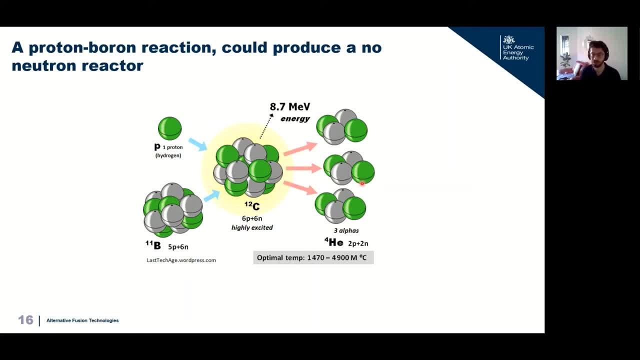 This potentially could produce a lone neutron reactor. You'll notice, from the sort of equation here you're putting proton and boron in on the left, Boron is slightly heavier element than we're used to with our other, our other fuels and this spits out three helium nuclei. You'll notice that there's no neutron, That thing we talked. 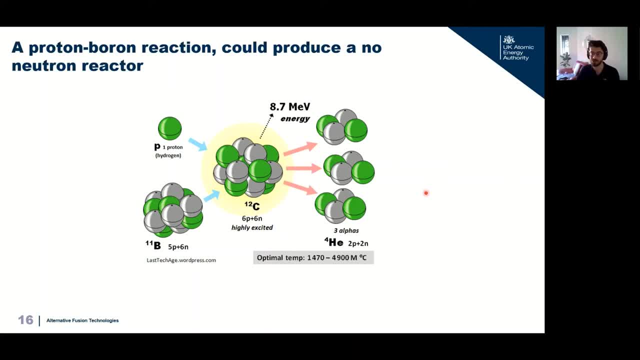 about in great detail and we've gone on in Fusion Tutorial 4 to talk about the problems that it causes. If you don't have a neutron, all of your resulting products just stay inside the plasma. You don't have so many issues about shielding. You don't have so many issues about remote handling. 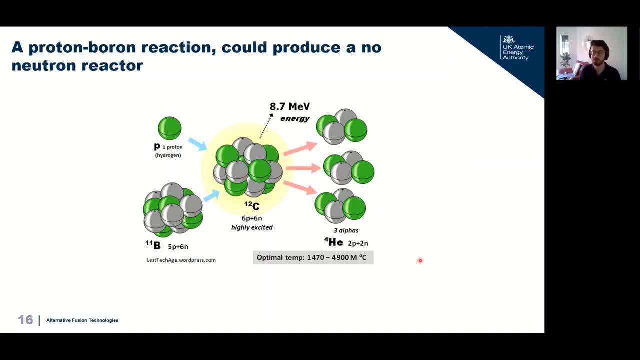 Now, further on in the cycle, some neutrons will be given out, so it won't be zero, but it'll be much, much less than our DT fuels. So potentially you can build a much simpler reactor overall, much cheaper, much smaller. The downside or the drawback is the optimal temperatures which you 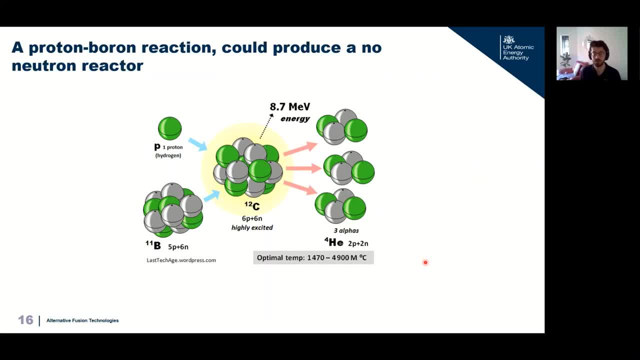 might have noticed from this diagram. So DT, we tend to run around 200 million degrees, which is pretty hot. I think we can agree they're fairly achievable with a fusion setup. Proton boron likes to be closer to one billion degrees. So a thousand million, potentially even higher. So that requires a very 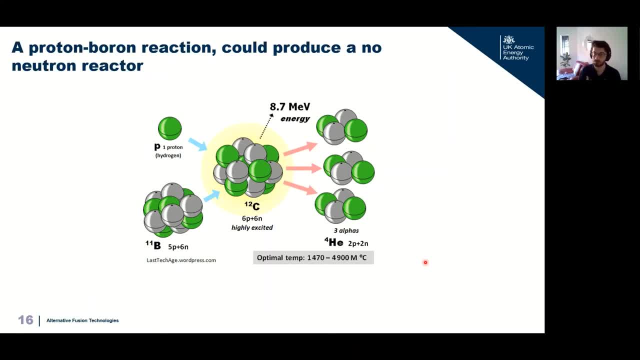 very, very high heating requirement. So not impossible by any means, but that's a big technological hurdle to come over. I've talked about a range of different approaches here, So to kind of preempt the question in your minds of you know which do I think is best. Well, 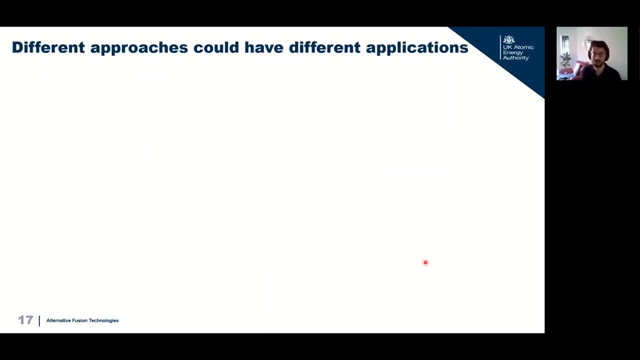 different approaches can have entirely different applications. If you think about the jet engine, it is the same core technology and, when used in different ways, can come up with entirely different applications. It's not to say any one of these is better or any others worse. They just have different pros and cons so they find different uses. Now, the same. 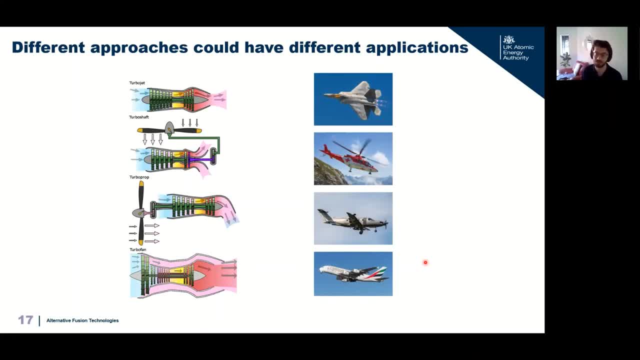 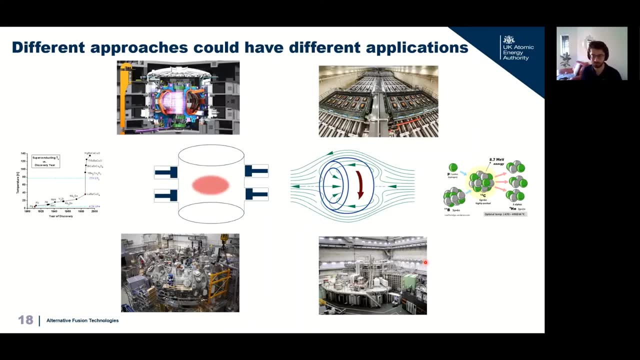 could be said potentially for future fusion technologies. And this variety of technologies is a very, very good example of a range of approaches. So the first one is the jet engine, The second one is the nuclear engine And the third one is the MED-2.. 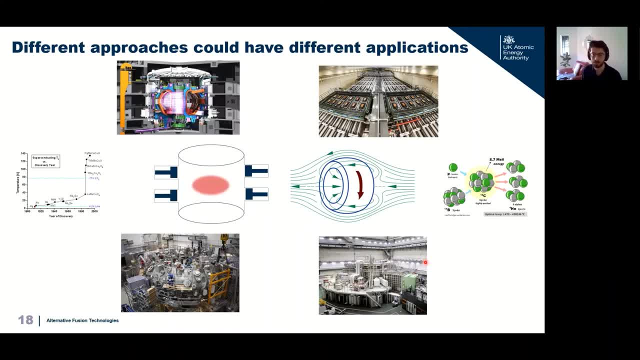 So these are very, very different approaches. So the variety of approaches is benefiting us in the short term too, because, exactly as we said with magnetic confinement research at the beginning, different approaches can lead to different solutions. It's this variety very positive for the field. It leads to a very healthy research environment and a very healthy. 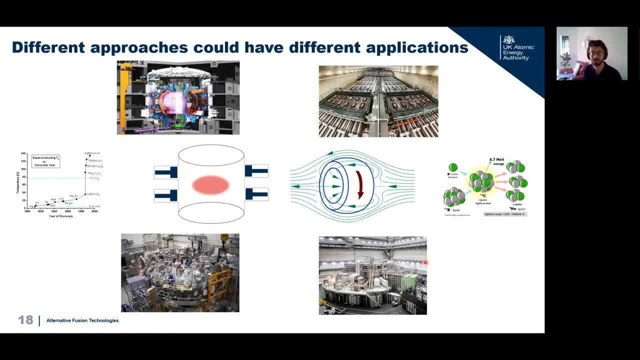 engineering environment, with the same benefits of the suppliers extending to the other technologies as well. Now I will say that tokamaks are still the most proven, They're the most mature of these technologies, and that's why we are continuing to pursue them. It's something we have a lot of expertise in as well. 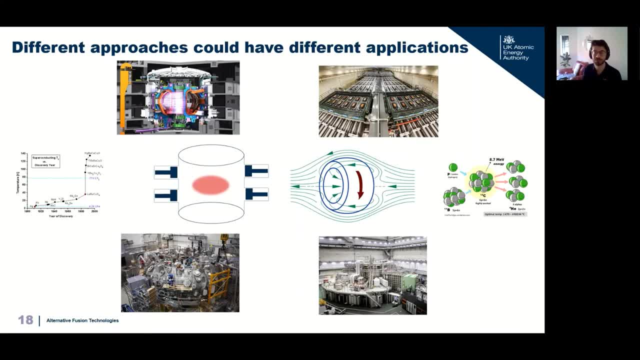 But these different benefits and drawbacks. we wish an absolute success to these other technologies and these are the things we want to encourage. We want the fastest route to fusion possible. Another benefit as well of some of these different approaches is it has seen a large increase in private investment in fusion. So on top of the government investment there's been around a billion dollars of private investment over the past five years. So overall creates a very healthy picture of fusion research going forwards. 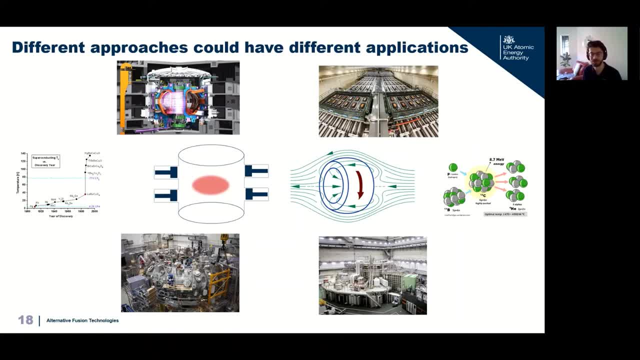 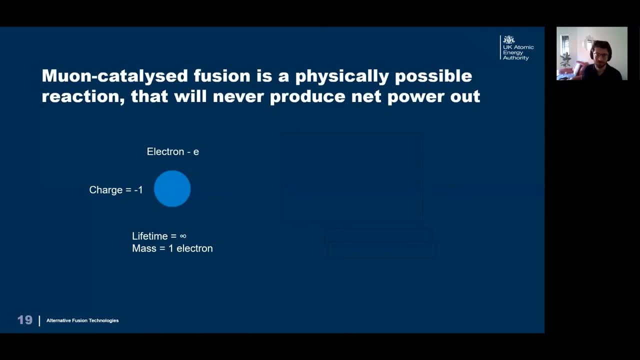 So at the end here I promised to answer a question about what's the new one. catalyzed fusion- It's pretty weird, Let's get into it. So muon catalyzed fusion, it's a physically possible reaction and it's never going to produce net power out. preface that at the beginning. 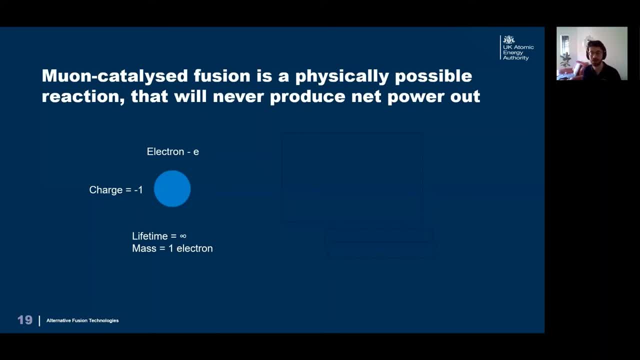 So it's another way of convincing a nuclei to fuse. Everything else we've talked about so far it's about getting them hot, getting it dense, getting it in there for a long time. This is completely different. So to talk about what muon catalyzed fusion is, I'll have to explain what a muon is first. 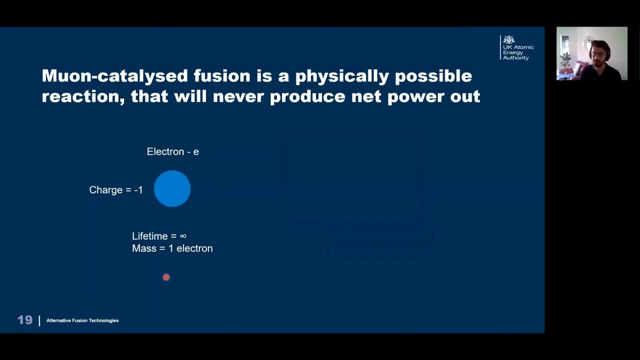 So we remind ourselves, muon is a very small particle because of the electron. Now, an electron is a fundamental particle, very small, negatively charged part of an atom. A muon is a similar particle in that it's also got a negative charge, so it can do the same jobs that an electron does, But a key difference and you can think of it kind of like an exotic electron. 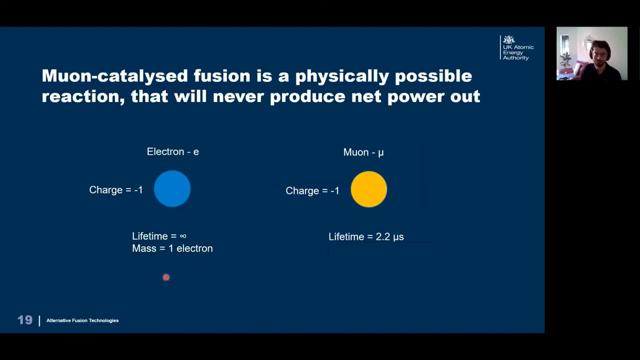 is that it decays very quickly, whereas electrons live forever. and it's much, much heavier. Its mass is 207 times the mass of an electron. So muon is a very small particle because of the electron. Now, an electron is a fundamental particle, very small, negatively charged part of an atom. 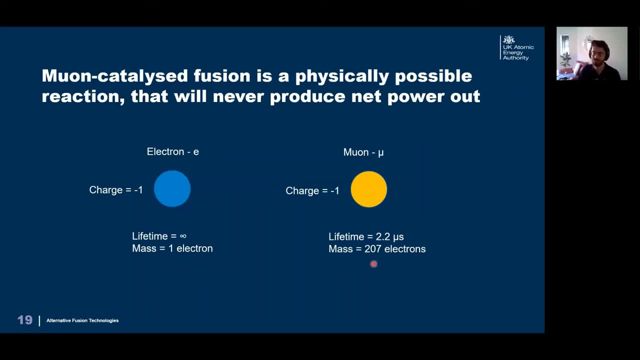 And its mass is 207 times the mass of an electron. So there are 207 times heavier in fact. So it's a very, very heavy electron that will disappear very fast. If you had a collection of them, 2.2 microseconds later, half of them had gone- another 2.2 microseconds, half had gone again. 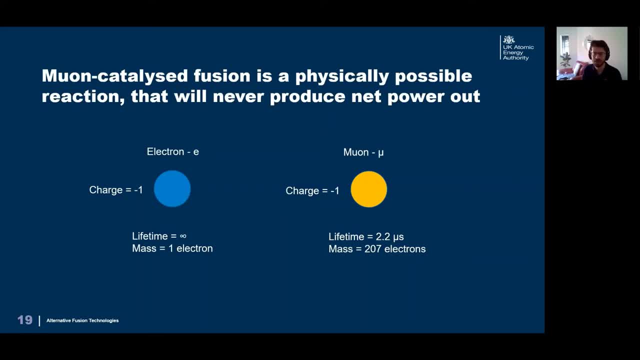 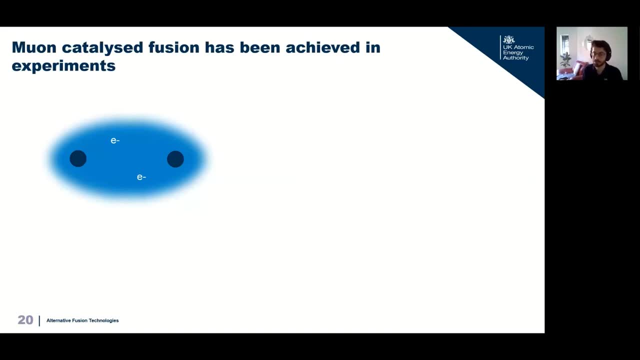 So they disappear very, very quickly. So they disappear very, very quickly. How on Earth is a heavy electron going to get us any felicent fusion So late on catalyzed fusion? if we think about a hydrogen atom, this is to the ocean. 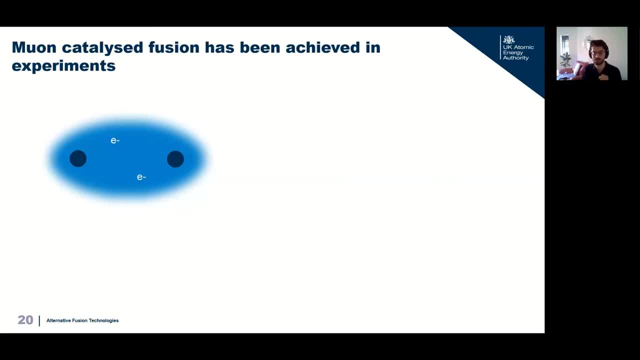 This is theلام of hydrogen material, the lumen of a atom. So muon catalyzed fusion worked like this when we first started CO2ing it: hydrogen atom, which is what we've got here. on the left we've got two nuclei. 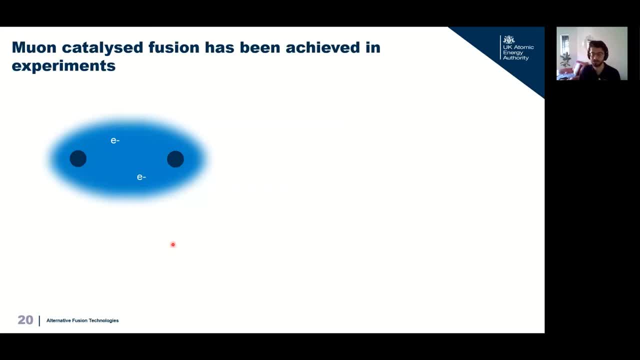 and they're bonded by two electrons. now you can artificially replace these electrons with a muon and if you do that, recall that the muons are 207 times heavier. that cinches the whole particle up and reduces its radius massively, way more than my PowerPoint animation suggests. it will reduce the radius by a. 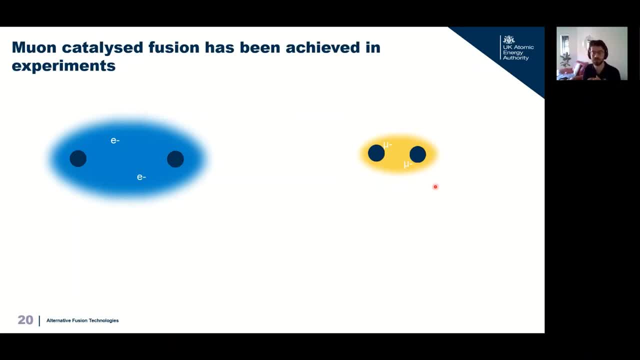 factor of 200. so suddenly now these two atoms in this molecule together are much, much, much closer together, and in their random vibrations they are much more likely to collide. this means that fusion can now happen at room temperatures even all the way down to cryogenic temperatures, which is actually where 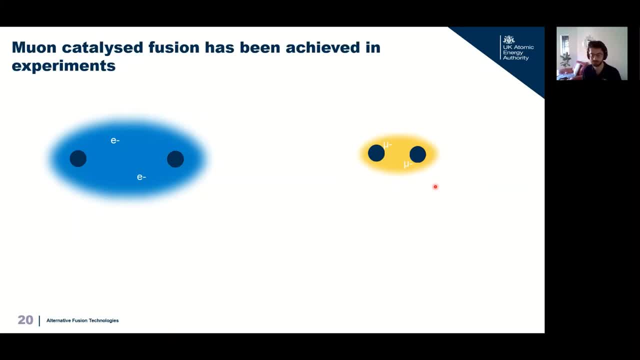 some of the experiments have been done at down close to absolute zero, and these very experiments have been done back in the 50s. so that's great. let's think about that. Let's go out, get some muons, build a muon catalyzed power plant. 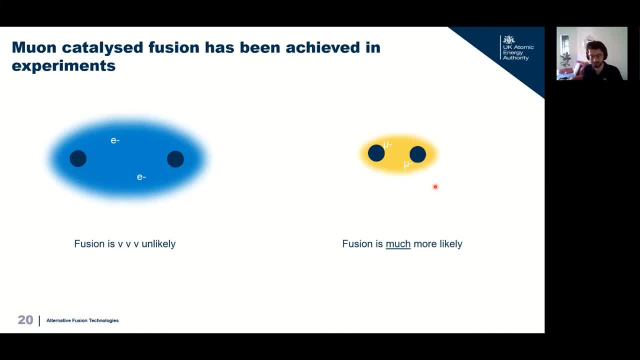 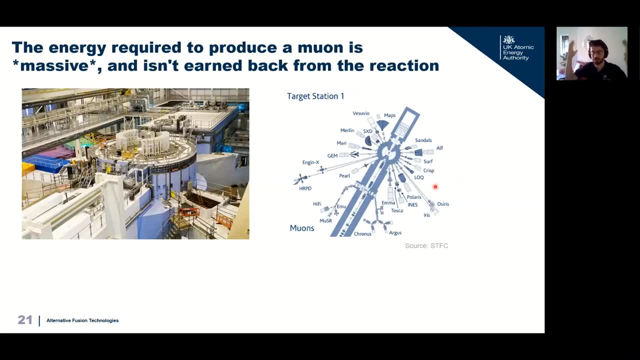 and, as I say here, this makes it so much more likely that it's going to happen. the issue comes with getting hold of the muons. they do occur, naturally. they happen in the upper atmosphere when solar radiation bombards it, and but they decay incredibly quickly and 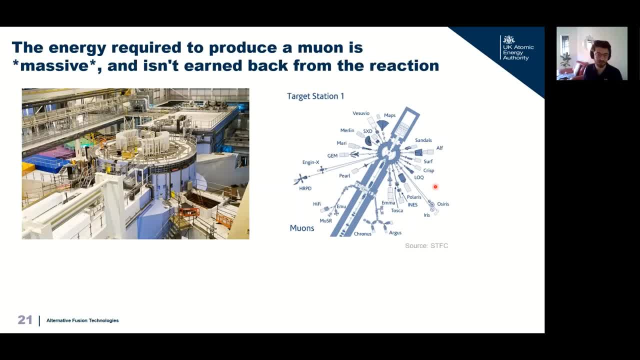 they've sort of gone by the time they've arrived. so it's possible to make them artificially. but it requires a part of a particle accelerator to create, just like the Isis accelerator over at Harwell, which is another scientific research campus based near ours at Cullom. so it's 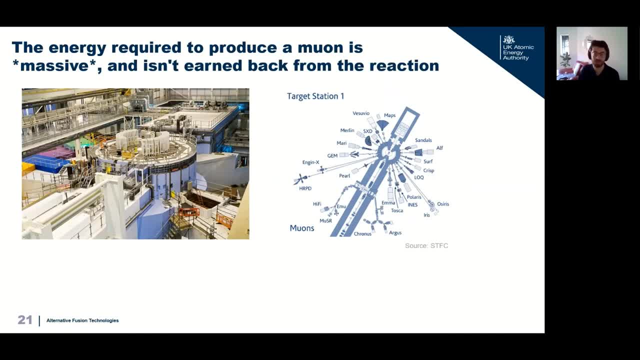 a very large particle accelerator and they produce muons as well as neutrons. so this is one of their target stations and you can see, here they've got these beam lines which are which they create muons on. The difficulty here is that for each muon it costs about five giga electron. 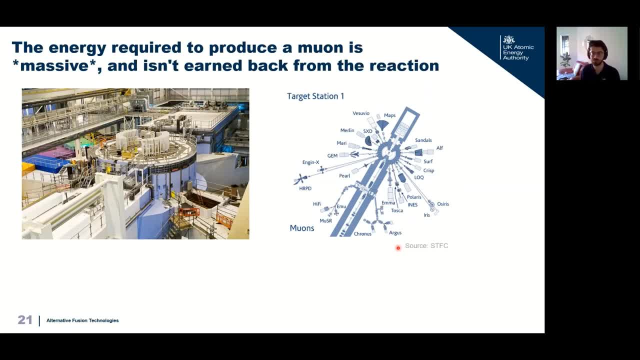 volts to create. don't worry about the units too much, but just remember this number five. now, when the muon goes on to catalyze fusion reactions, the most energy you can get out. on average it's going to be 2.7 giga electron volts now. 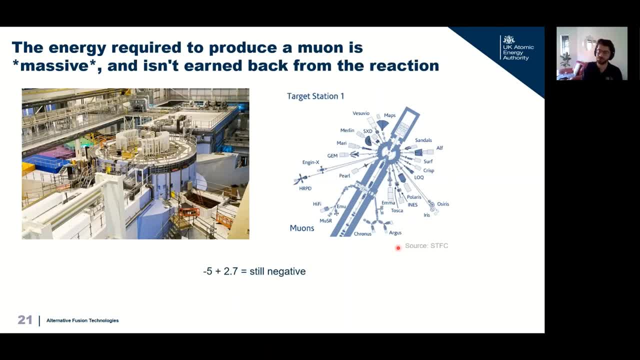 it's apparent straight away. you put in five, you've got out 2.7. that's still a negative number. there's just no way of making that come out positive. so yes, muons are useful for science. Isis actually use them for imaging. they send a beam of muons through objects and they can look through them without damaging. 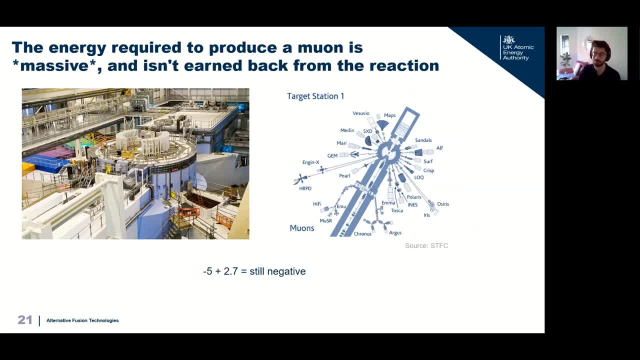 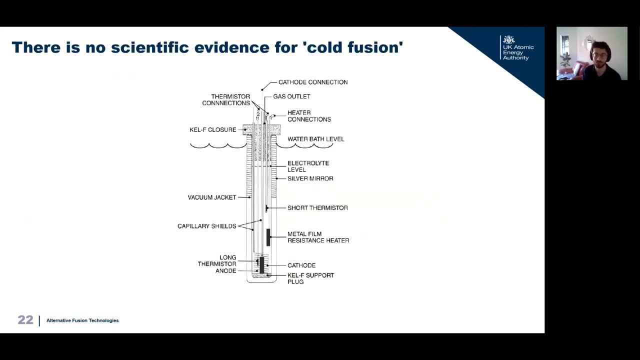 them, but unfortunately that reaction is never going to prove useful for creating power out. Now, whilst we're talking about fusion happening at conditions that are not hot, it's worth paying mention to cold fusion. So cold fusion is a term usually used to describe an experiment by professors Fleischmann.